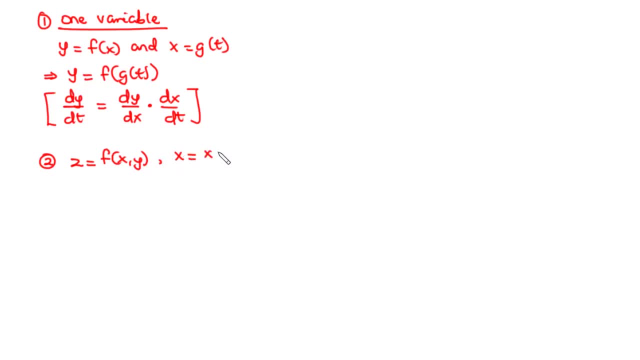 So we have x to be equal to x of t, And then we have y also to be a function of t. that is y of t. Now, with this, the composition z equals f of now, in place of x, we have x of t. In place of y, we have y of t. So the composition that is being expressed as z equals f of x of t, y of t. 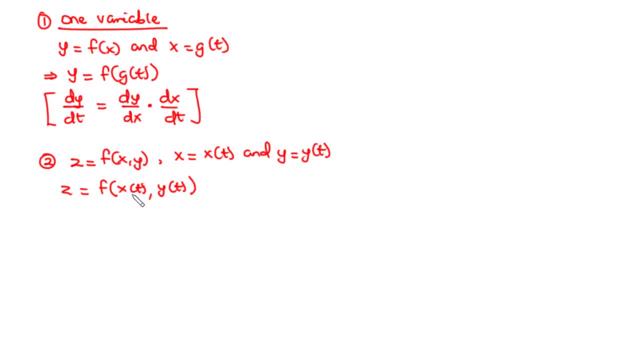 expresses z as a function of a single variable, t. Therefore, we will need to find dz dt. We will need to find dz dt And to find dz dt, we need four components. We need four components, which are: we need the partial derivative of z with respect to x, partial derivative of z with respect to y. 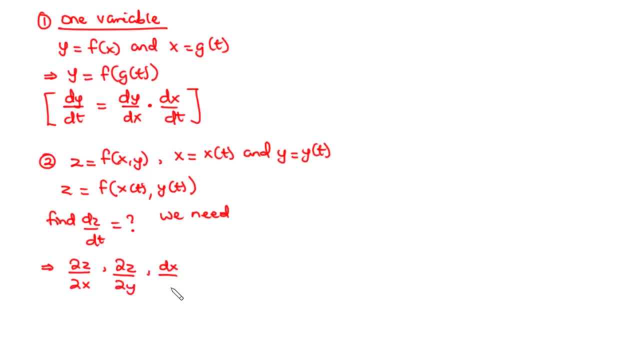 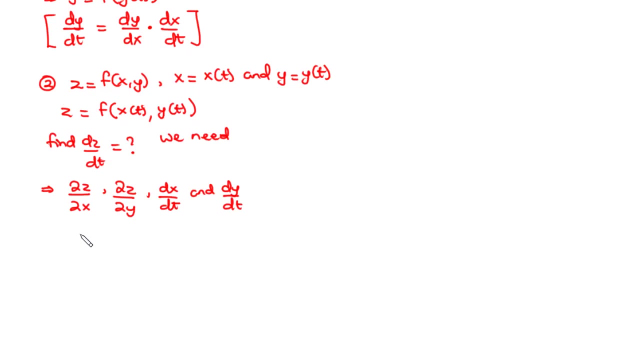 The first derivative of x with respect to t, as well as the first derivative of y with respect to t. Now we can think of this as having a tree diagram. So with a tree diagram we have z as the dependent variable that is on top, And then z is a function of two variables: x and y. 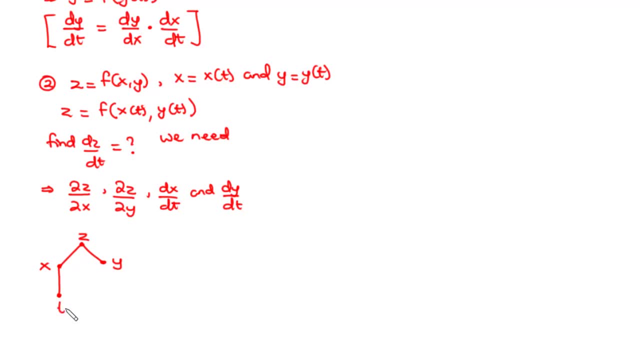 And then x is a function of two variables- z and y. And then z is a function of a single variable, t. y is also a function of a single variable: t. Now to move from z to x and then z to y. Since z is a function of two variables, to move from z to x, we need the partial derivative of z with respect to x, And then, to move from z to y, we need the partial derivative of z with respect to y. 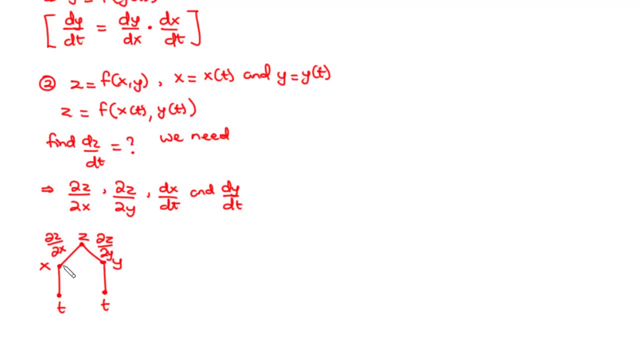 The reason why we need the partials with respect to x and y is simply because z is a function of two variables, and then to move from x to t, because x is a function of a single variable, we basically need the x, the t, same for y: we need the y. 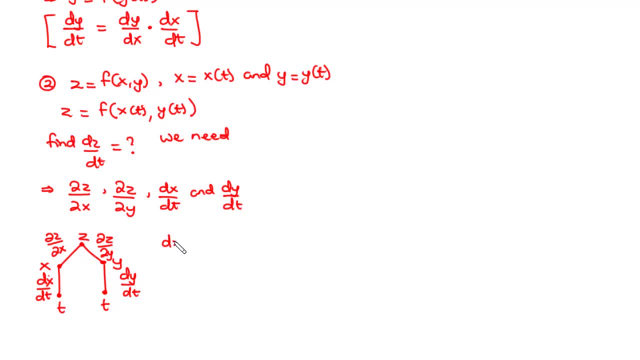 the t. therefore, to find the z, the t, the z, the t is given by the partial derivative of z with respect to x times the x, the t, plus the partial derivative of z with respect to y times the y, the t. basically, this is the chain rule formula for functions of two variables. 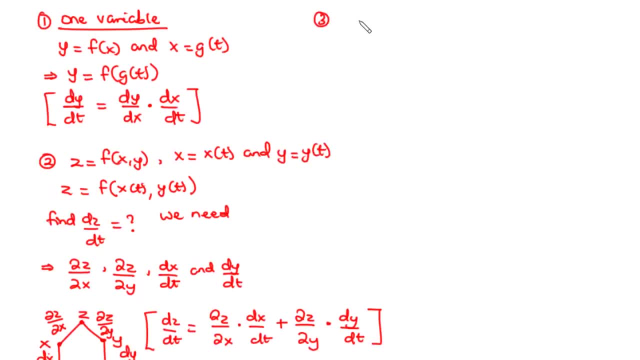 now let's move on to functions of three variables. so, given that w is a function of three variables- x, y- Now lets set x as the express derivative of the uh, the x. hope you 97 unconditionally liked the video. Thank you, Bye. 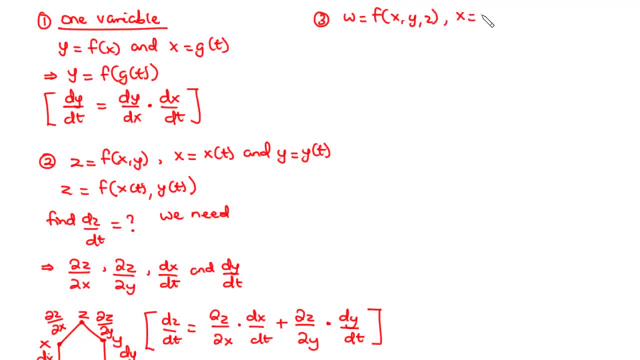 and then z, and then x is said to be equal to x of t, y is equal to y of t, and then z is also equal to z of t. thus x, y and z are all functions of t. then we can find, we can find the w, the t, and that is given by: we have the partial of w with respect to x times the x, the t. 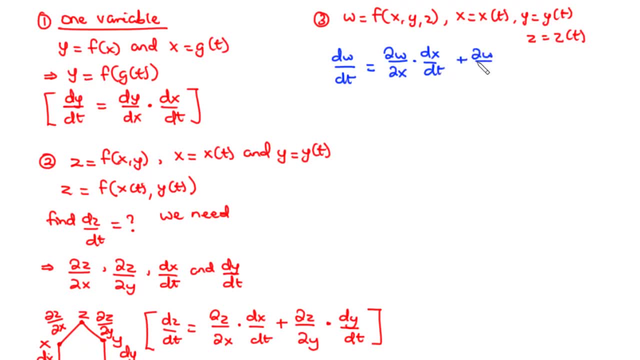 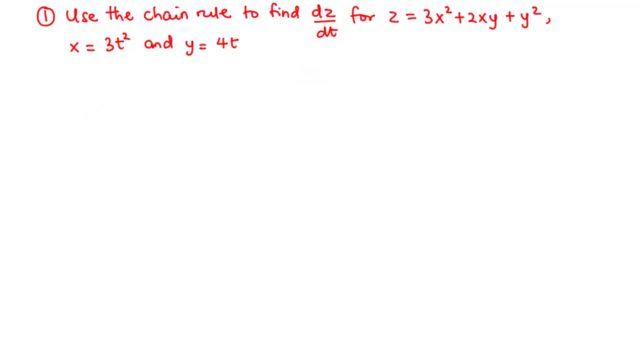 plus the partial of w with respect to y times the y, the t, plus the partial of w with respect to z times the z a t. so basically, this is the chain rule formula for functions of three variables. now, at this point, let's consider some examples. so let's take our first example in our first 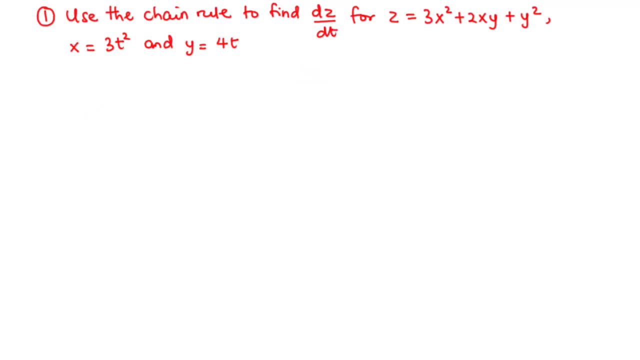 example, we are going to use the chain rule to find z, dt, for z equals 3x squared plus 2xy plus y squared, where x is equal to 3t squared and then y is also equal to 4t. now you realize that z, here the function, z is a function of two variables: x and y. 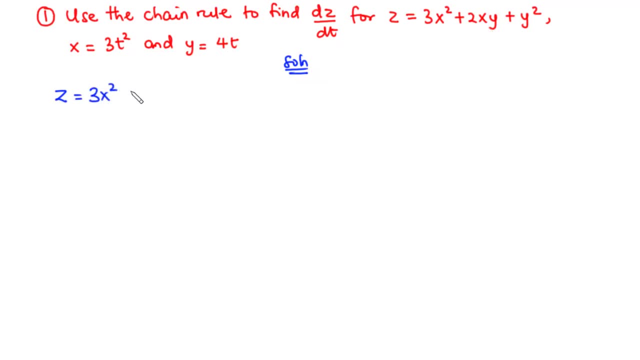 now we have z to be equal to 3x squared plus 2xy plus y squared, and then we have x and y to be functions of a single variable, t. so x is equal to 3t square, and we have y also to be equal to 4t. 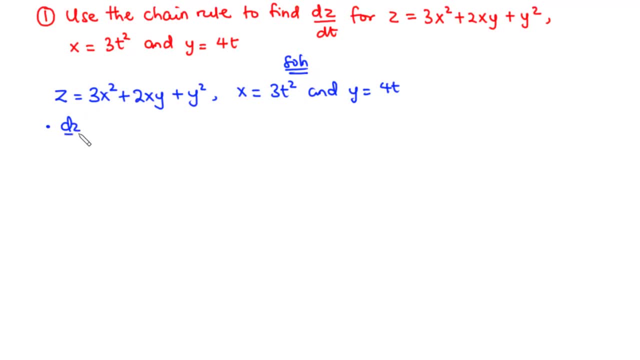 now to To find dz dt. we know that that is equal to the partial derivative of z with respect to x times dx dt, plus the partial derivative of z with respect to y times dy dt. So we need to find partial with respect to x, partial with respect to y dx dt, and then 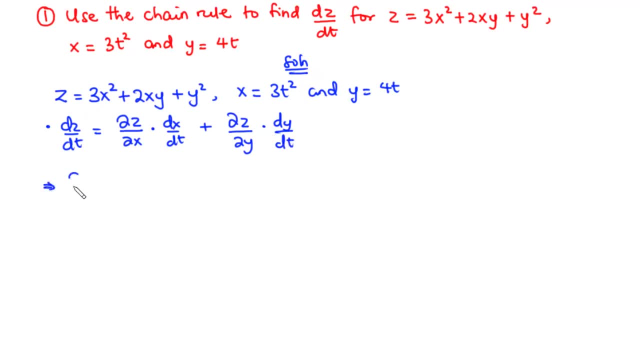 dy, dt. So first, the partial derivative of z with respect to x means that we are going to differentiate this function, that is, z with respect to x. So in doing so we are going to keep y constant. So for the first term we have 3x square. we differentiate that with respect to x and 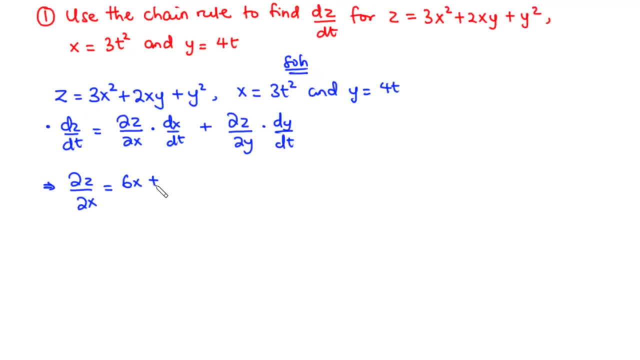 then we have 6x plus. we are going to keep y constant. We differentiate 2x. We are going to keep y constant. We are going to keep 2x with respect to x, and then we have 2.. So we multiply that by y and that becomes 2y. 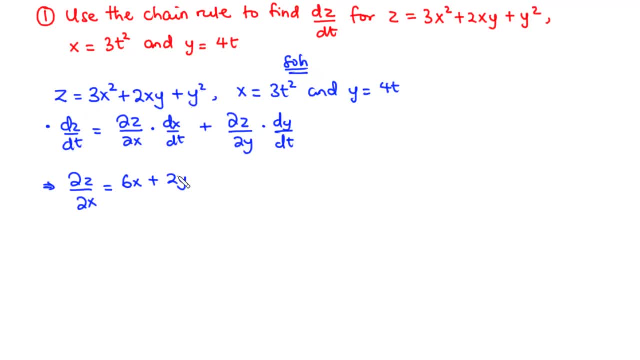 Now, because y square is a constant, we differentiate that and then we get 0.. So we have our final expression to be 6x plus 2y for the partial derivative of z with respect to x. Now we know that x is equal to 3t square and then y is equal to 4t. 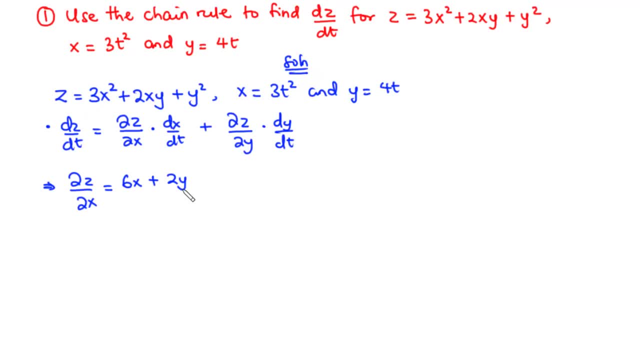 So we are going to substitute the expressions for both x and then y into 2.. So in doing so, we are going to keep x as constant for z and then h as constant for z. This is going to be I times 2.. 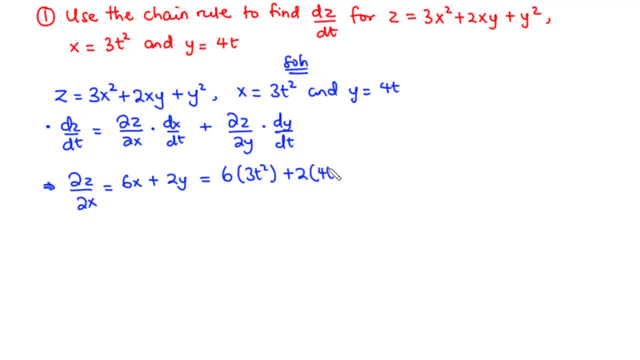 So we multiply both x and y to get 6.. So now we have 6 values of z with respect to y, and x is equal to 2t plus 9t. That sums up the 2 function to be equal to 3t. 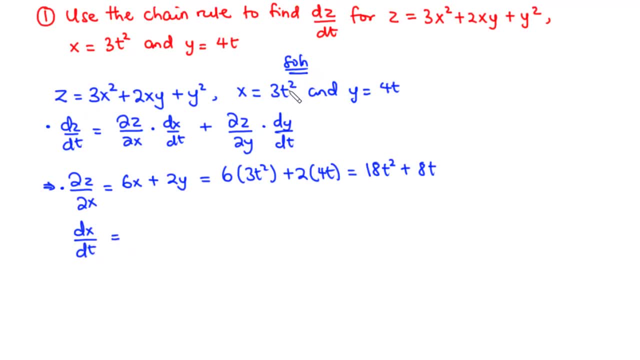 We also know the 2 function Southwest. So we know Xen is equal to 0. So 5 times X add up to 50. That is change the denominator toankers So that becomes 60. And then we move on to the partial derivative of z with respect to y. 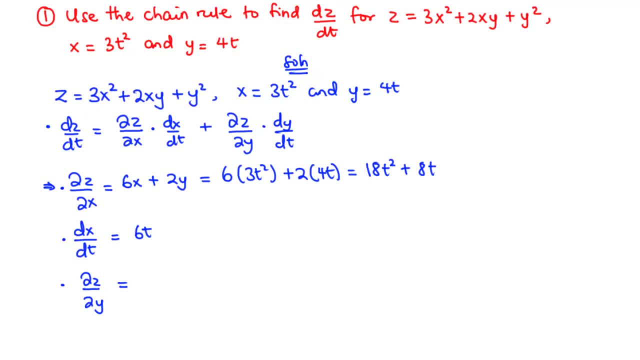 We are going to differentiate this same function with respect to y. So 3x squared is a constant. It goes to 0 after we differentiate it And then we move on to 2xy. We are going to keep x constant and then we differentiate to y. 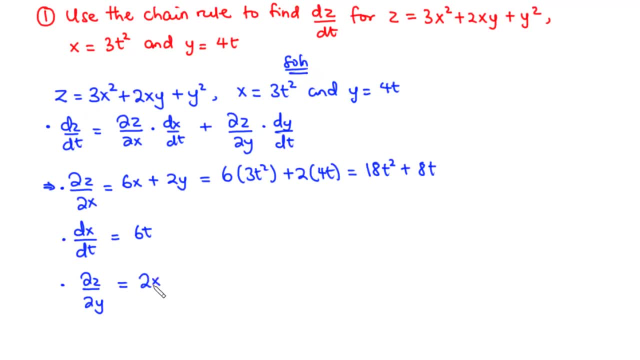 And thus we have 2.. So that becomes 2 times x, plus we differentiate y squared, We have 2y, And thus we substitute the expressions for x and y in here, So that we have 2 times 3t squared plus 2 times 4t. 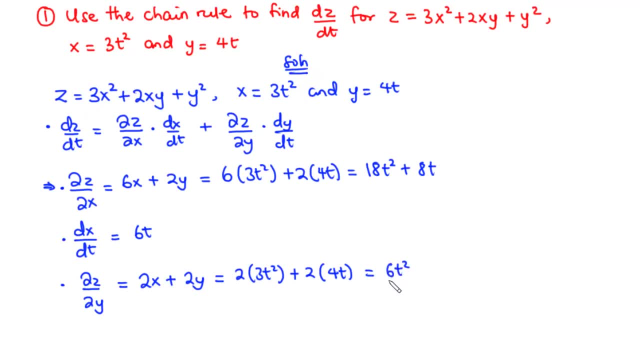 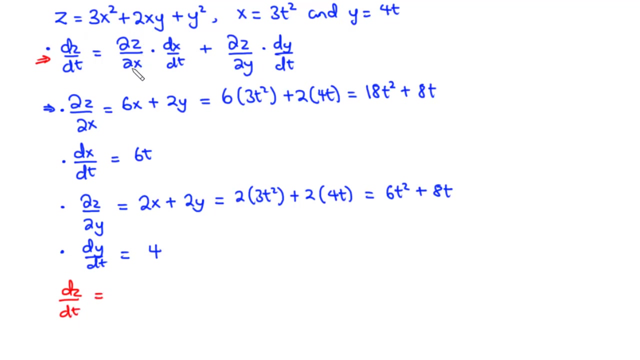 So this becomes 6t squared plus 8t, And then We want to find the y, the t, So that will be equal to 4.. So, finally, we are going to substitute these expressions in here So that we have the z, the t, to be equal to partial of z with respect to x. 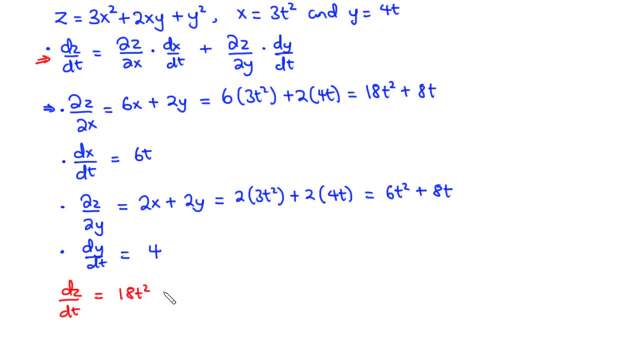 That is 18t squared plus 8t. So you multiply, You multiply that by the x, the t, and that is equal to 6t plus we have partial with respect to y, that is 6t squared plus 8t. and then we multiply that by the y, the t, which is 4.. 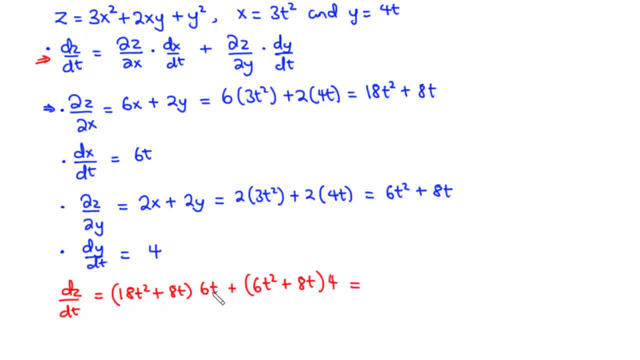 So we are going to have 18 times 6.. That is 108.. And then t squared times t, That is t cubed plus 6 times 8. We have 48.. And then t squared plus 4 times 6, 24.. 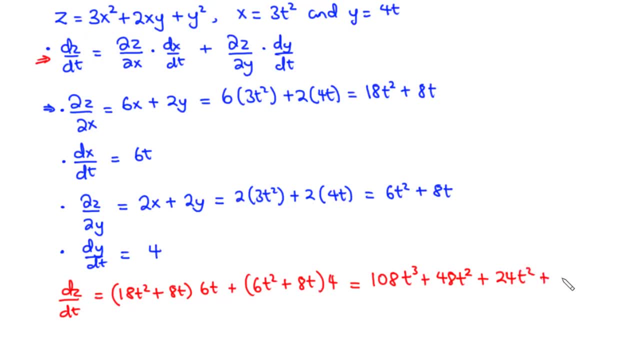 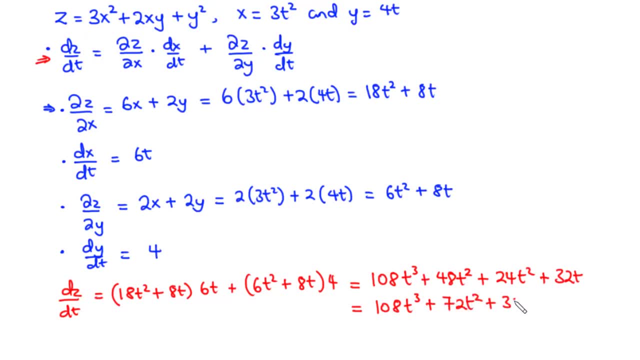 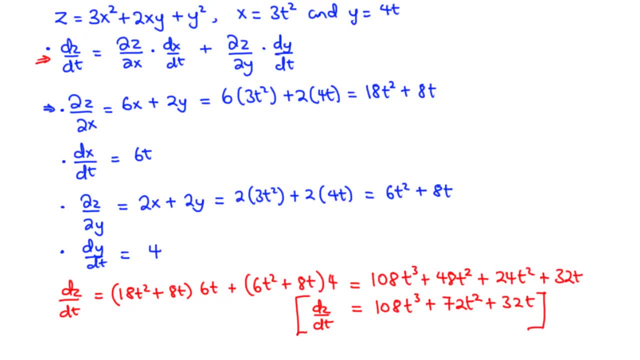 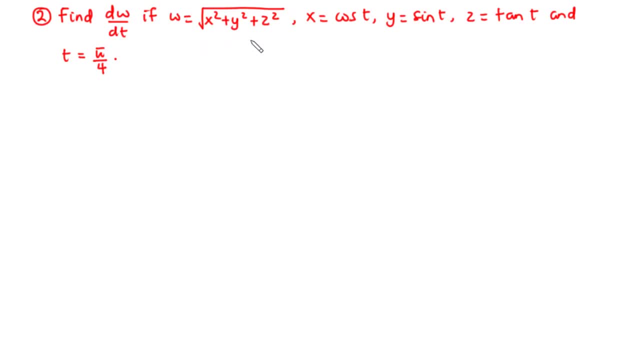 So now let's move on as we take the second example. Now to example 2, we are going to find the w? dt. If w is equal to the square root of x squared plus y squared plus z squared, x is equal to cos t, y is equal to sin t, z is equal to tan t. 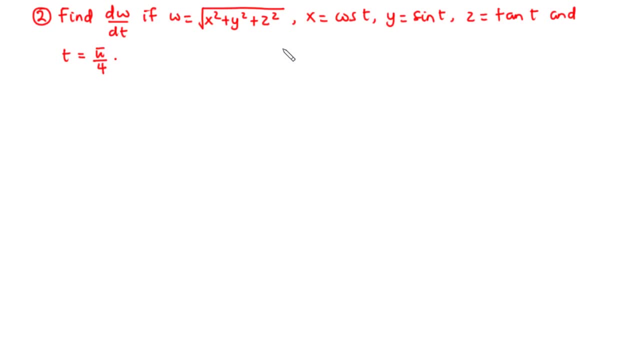 and then t. So t is given as pi on 4.. So let's try this together. So we have w to be the square root of x squared plus y squared plus z squared. We can express this as x squared plus y squared plus z squared, all exponents 1 over 2.. 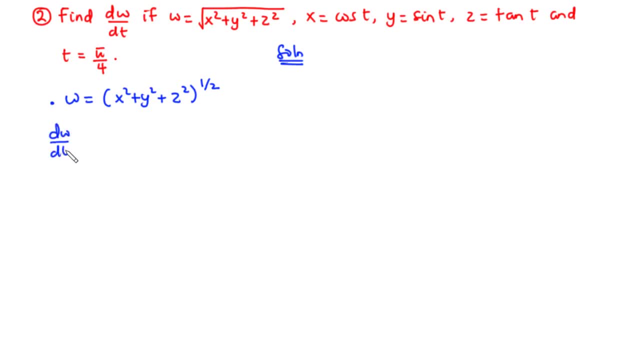 Now to find the w dt. we know that is equal to the partial derivative of w with respect to x. So we have w times dx dt, plus the partial derivative of w with respect to y times dy dt, plus the partial derivative of w with respect to z times dz dt. 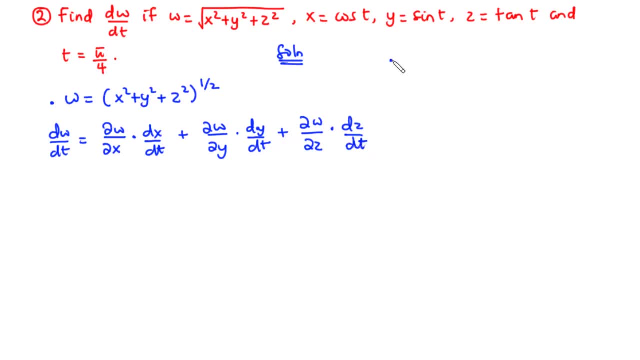 Now, even before that, let's try to simplify these three. That is x, y and then z. Now we know that x is equal to cos t, And then t is given as pi on 4.. So automatically we have cos pi on 4, and then that is equal to cos 45.. 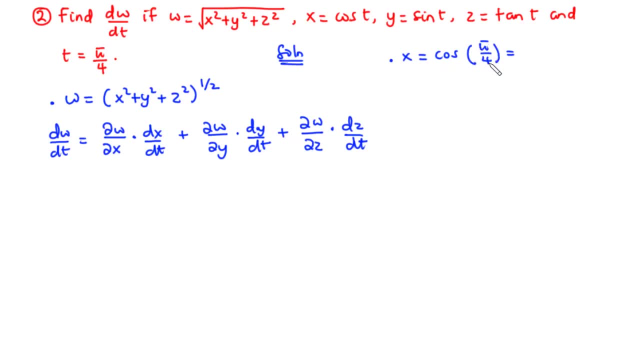 So if you want to evaluate this cos pi on 4, your calculator should be in the radian mode. If you want to express pi in degrees, that is 180 divided by 4, and that will be 45. Therefore, cos 45, your calculator should be in the degree mode. 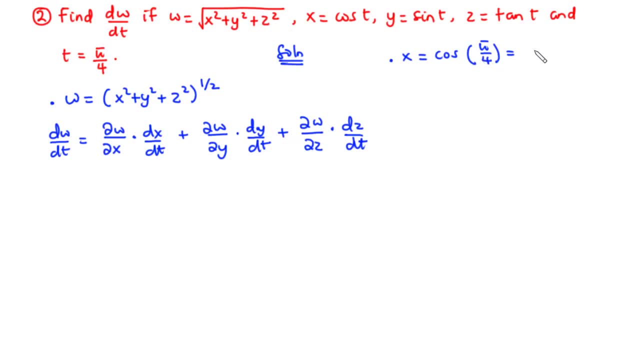 So cos 45, or cos pi on 4, is equal to 1 over root 2.. y is equal to sine pi on 4,, and that is also equal to 1 over root 2.. And then z is equal to tan pi on 4,, and that is equal to 1.. 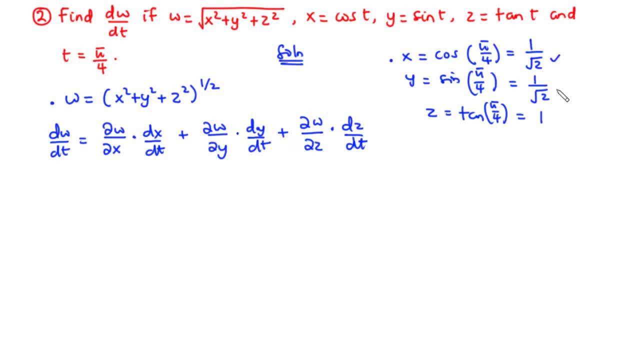 So we should take notice of these three. So we should take notice of these three. Now let's try to find the partial derivative with respect to x. So we have partial derivative of w with respect to x and that is equal to so considering. 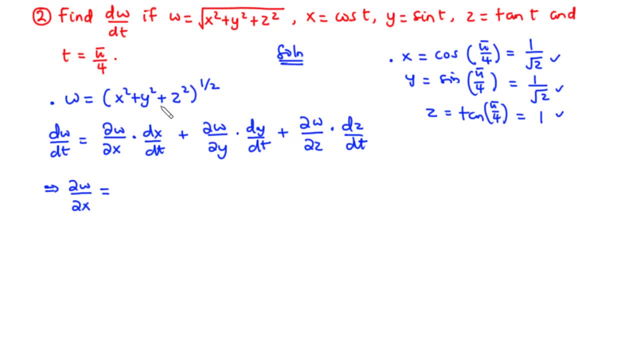 this function, we are going to use the shortcut form of the chain rule to find the partial derivative with respect to x. So basically, we are going to drop down the exponent. We differentiate x square, we have 2x. notice that we keep y and then z constant. so there. 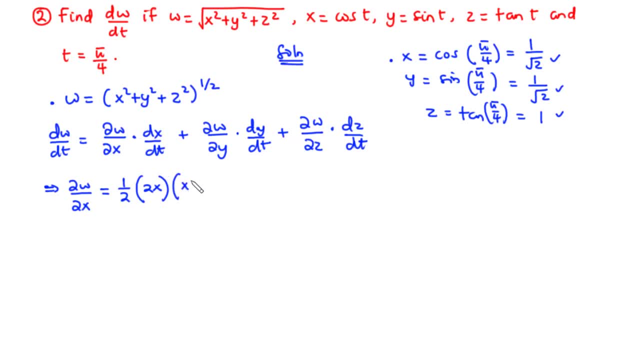 the derivative go to 0. We are going to repeat what we still have in the bracket and then we are going to reduce the exponent by 1.. So that is negative 1 over 2, exponent negative 1 over 2.. So 2 cancels out 2, we are left with x. 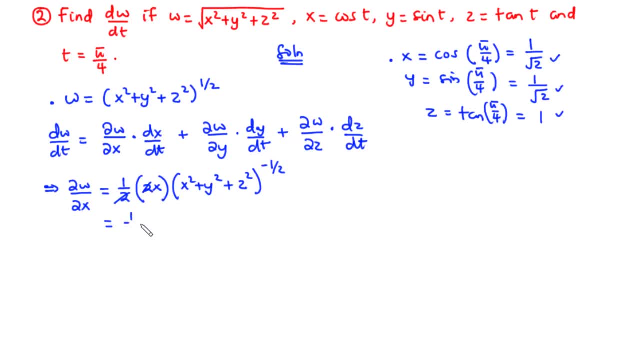 Now x here is said to be 1 over root 2.. So we have 1 over root 2.. 2 times x square, that becomes 1 over root 2 r square plus y square: 1 over root 2 r square. 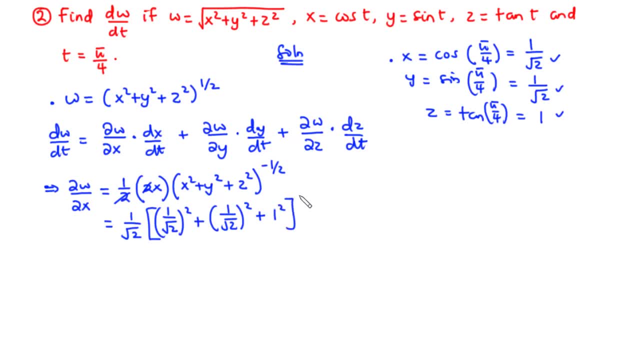 plus z square, which is 1 square, All exponents negative, 1 over 2.. So we have this to be 1 over root 2. into brackets: 1 square is 1, root 2 square is 2.. So this becomes 1 over root 2 times half plus half is 1, plus 1 is 2, so 2 to the power. 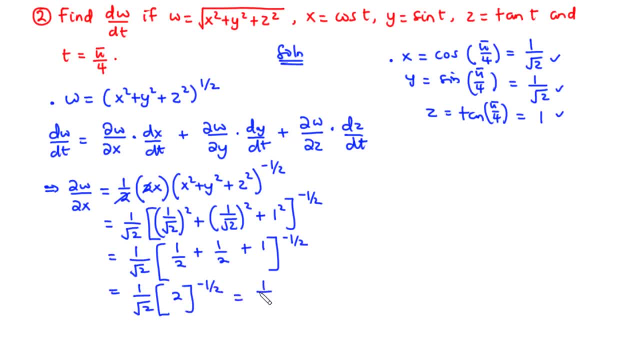 negative 1 over 2.. So this becomes 1 over root 2 times now, because we have a negative here, it suggests that we have 1 over 2.. Square root of 2.. So this finally becomes 1 over 2, because square root of 2 times square root of 2 is equal. 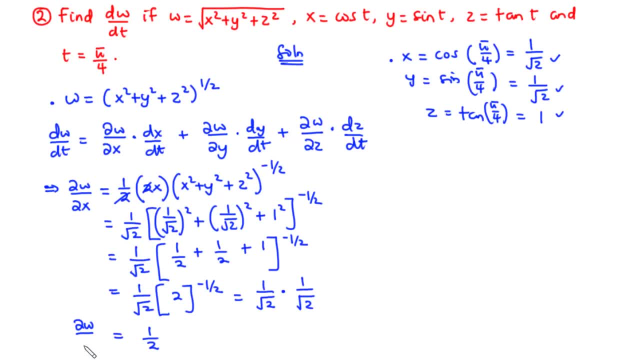 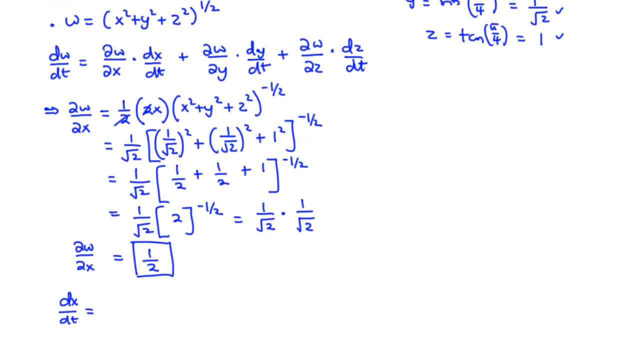 to 2.. Therefore, the partial derivative of w with respect to x is equal to 1 over 2.. Now let's move on as we try to find the x dt. So we have x. We have x to be equal to cos t. 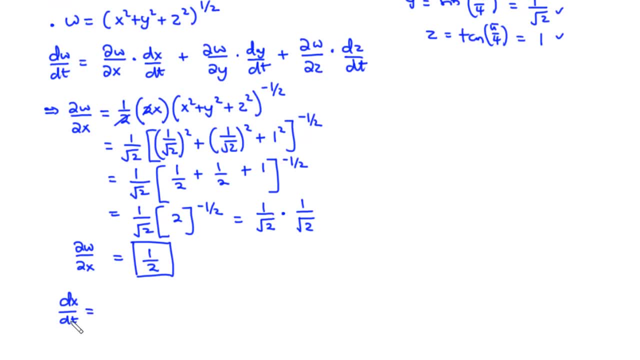 Therefore, therefore, the x dt is equal to negative sine t, And that would be equal to negative sine pi on 4, and that is equal to negative 1 over root 2.. So this is the x dt. Now move on to partial derivative of w with respect to y, and that will be equal to. so for this same. 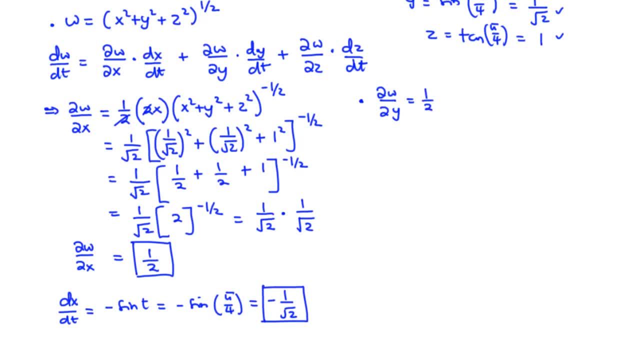 function. we drop down the exponent, we differentiate what's in the bracket with respect to y. we have 2y. we are going to repeat what we have in the brackets and then we are going to reduce the exponent by one. so this is equal to: so two cancels out two. we have y and then y. here is 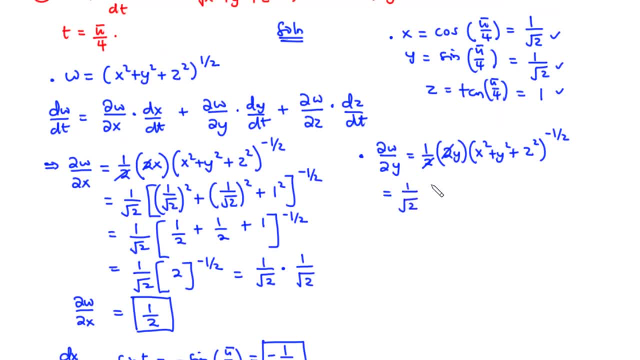 one over root two. so we have one over root two times one over root, two all square plus one over root, two all square plus one square. so we can basically ignore all those processes and then simply have two inside the bracket exponent negative one on two. so this is equal to one over root two times one over root two and that is equal to one over two. 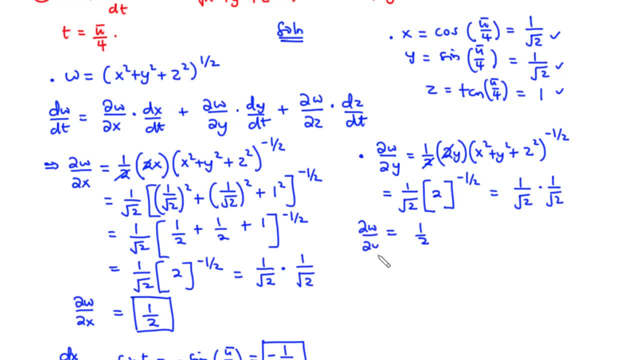 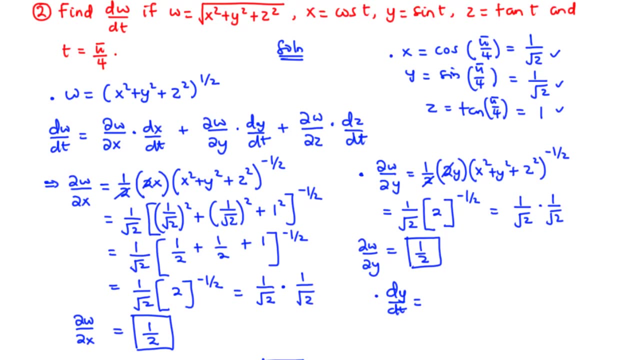 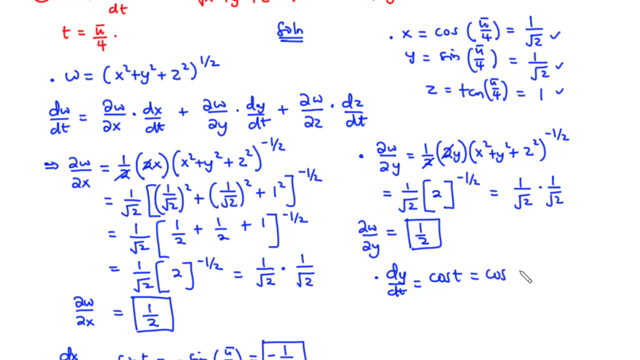 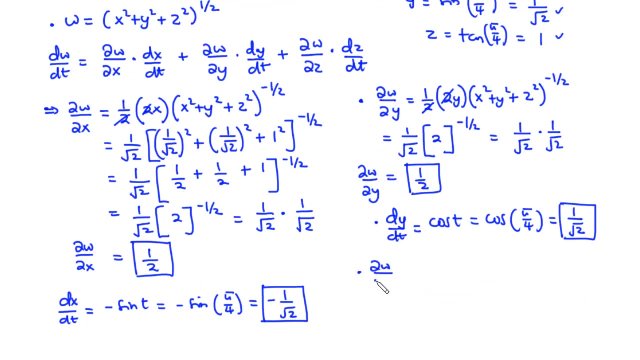 so you have the partial with respect to y also to be one over two. and then for dy a t, we have y to be equal to sine t, so dy dt becomes cos t, and that is equal to cos pi on four, and that is one over root two. so that is dy dt. now for partial derivative of w with respect to z, for the 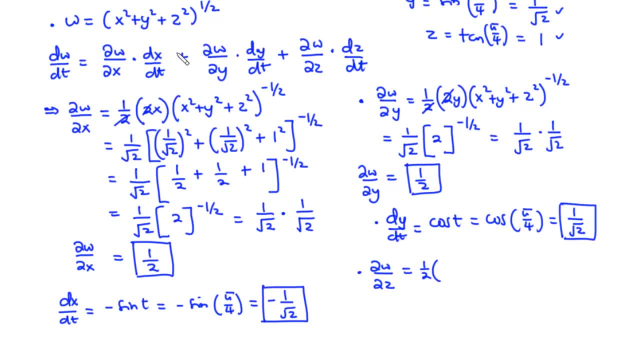 function. we drop down the exponent one over two. we differentiate z square. we have two z. we have x square plus y square plus z square. all exponents negative. one over two. two cancels out two. we have z to be equal to one. so one times. now notice that. 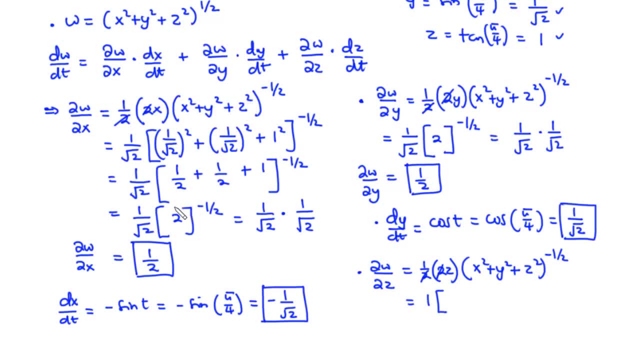 x square plus y square plus z square is what gives two. two raise to the power negative, one on two, so that becomes one times one over root two and that is equal to one over root two. so that is the partial derivative of w with respect to z. next we need to find the z, the t, so we have z to be tan t, so the z dt becomes. 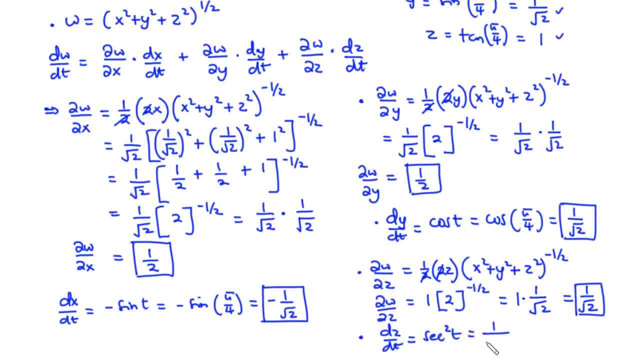 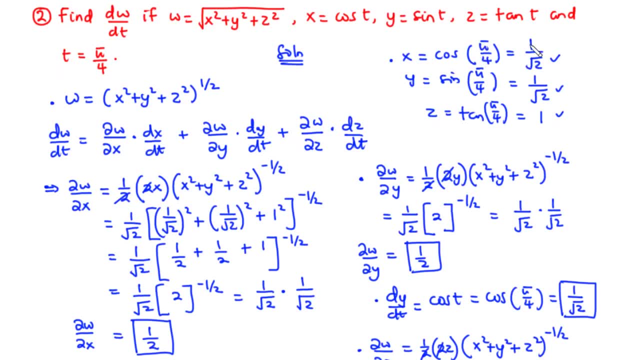 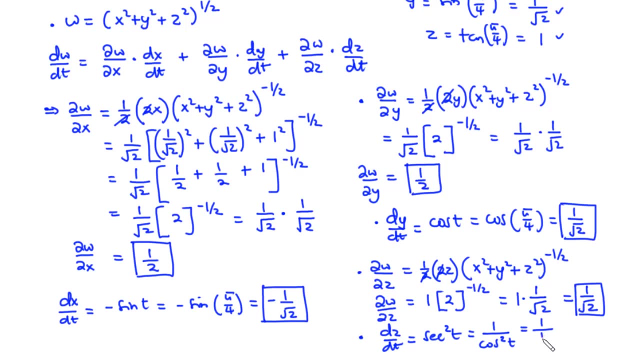 sec, square t, and that will be one over cos, square t, now cos t, cos t is said to be one over root two, one over root two. so finally we have this to be one over one over root two, or square simply because of the square here. so this becomes one over one. square is one, root two, square is two. 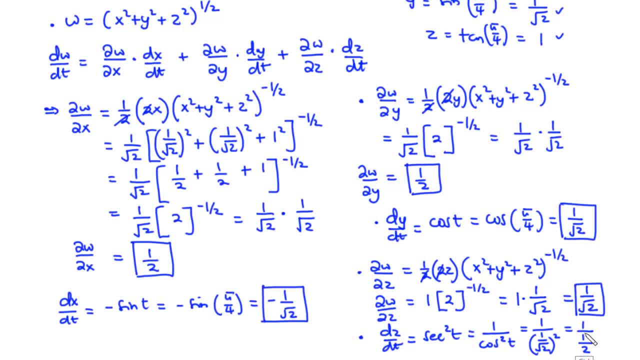 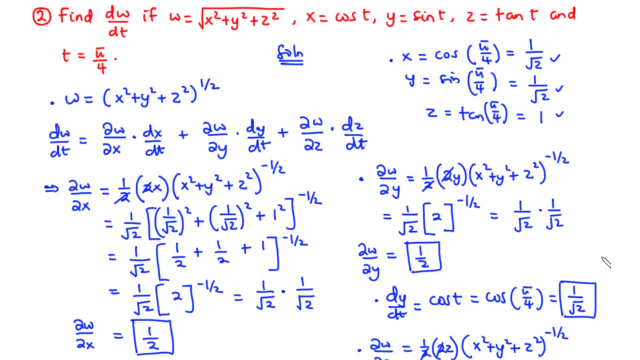 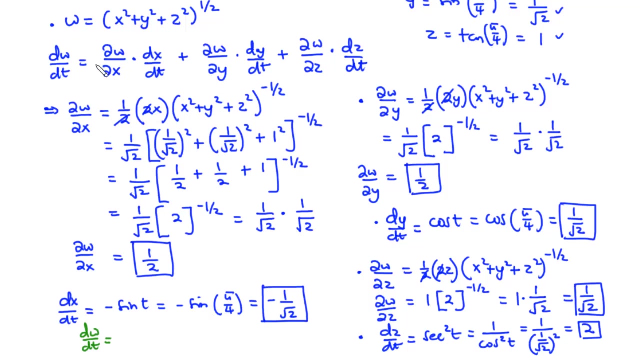 so that's finally going to be one times two over one, and that is equal to two. therefore, we have the z? dt to be equal to two. so finally, finally, we have the w? dt, so the w, the t, and that's equal to partial. with respect to x, we had that to be 1 over 2. 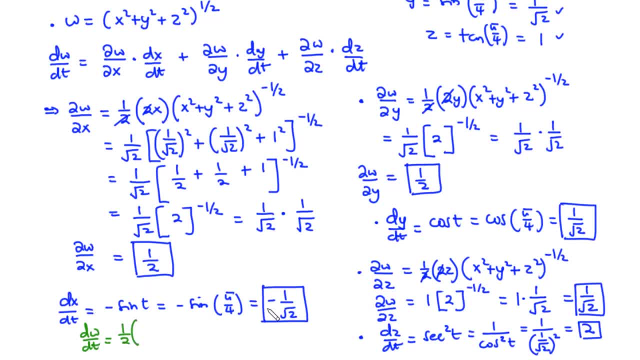 times the x dt, that is negative 1 over root 2, plus partial with respect to y, that we had 1 over 2. also times dy dt, that is 1 over root 2 again, plus partial with respect to z, that also we had 1 over root 2 and that is negative 1 over root 2.